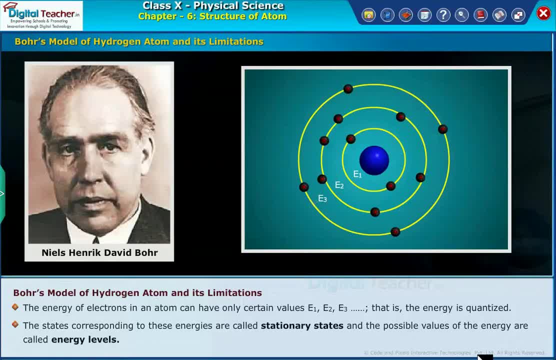 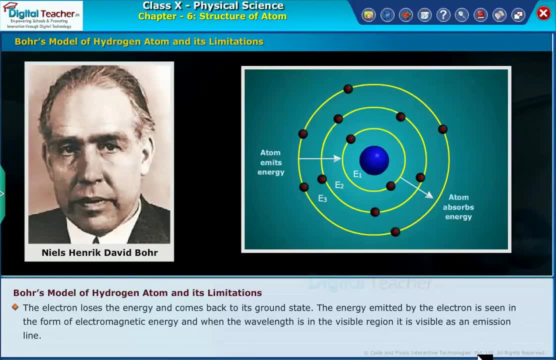 and the possible values of the energy are called energy levels. The electron losses the energy and comes back to its ground state. The energy emitted by the electron is seen in the form of electromagnetic energy and when the wavelength is in the visible region, it is visible as an emission line. 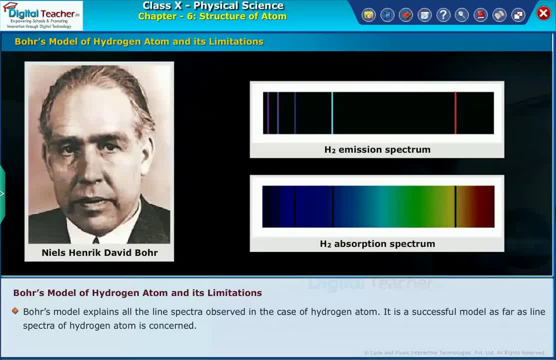 Bohr's model explains all the line spectra observed in the case of hydrogen atom. It is a successful model as far as line spectra of hydrogen atom is concerned. But the line spectra of hydrogen atom, when observed through a high-resolution spectroscope, appear as groups of finer lines. 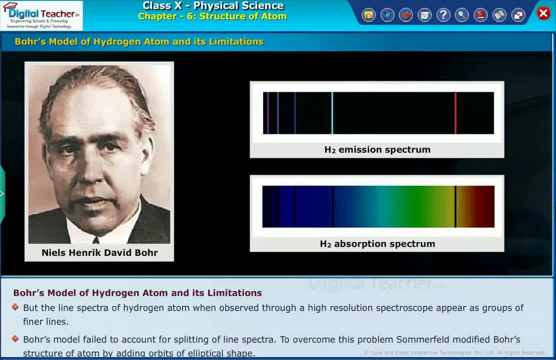